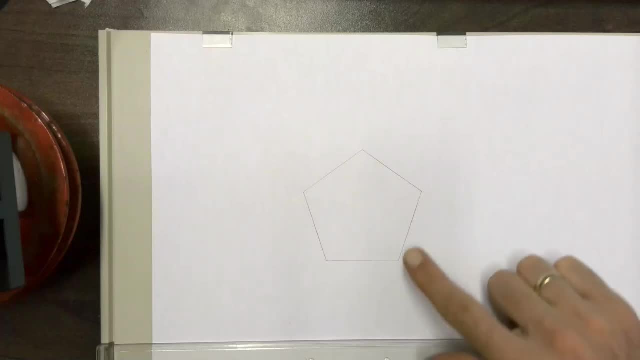 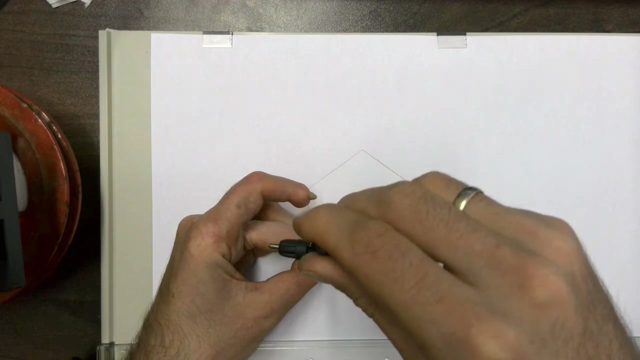 To find the center point of an already given pentagon. we use our set square method that we would normally use to construct the pentagon. So you'd start by bisecting the baseline of your pentagon by placing your compass on the one base end, opening it up to the other base. 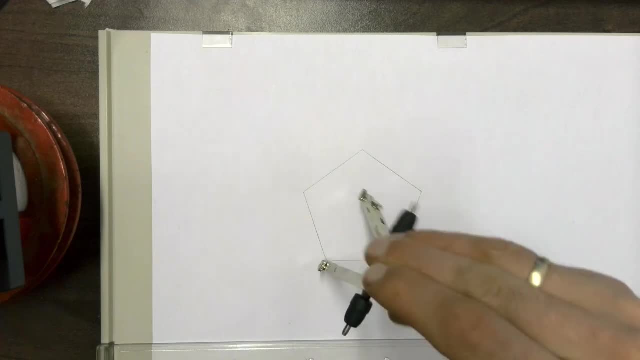 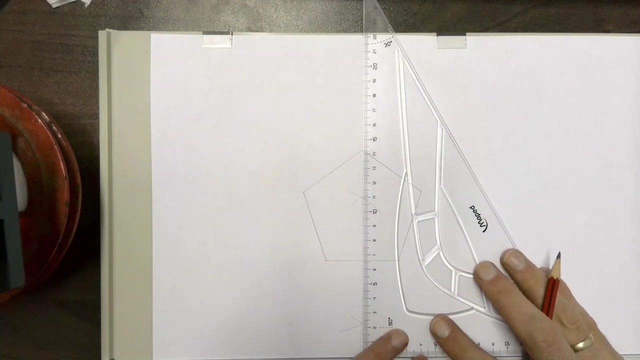 end and then drawing an arc on the top and at the bottom, Flip your compass around, place it on the other base end, draw another arc at the bottom and at the top, Take the intersection point between those sets of arcs and draw a construction line. Take your 60 degree set. 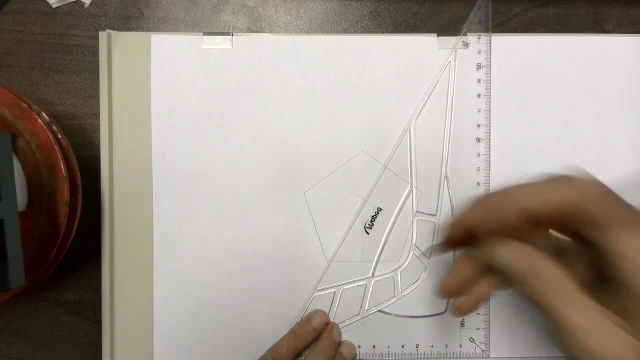 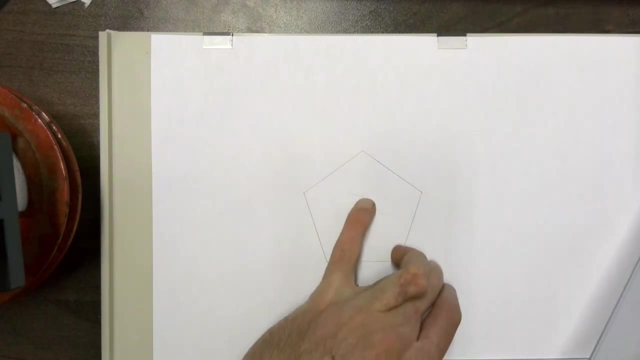 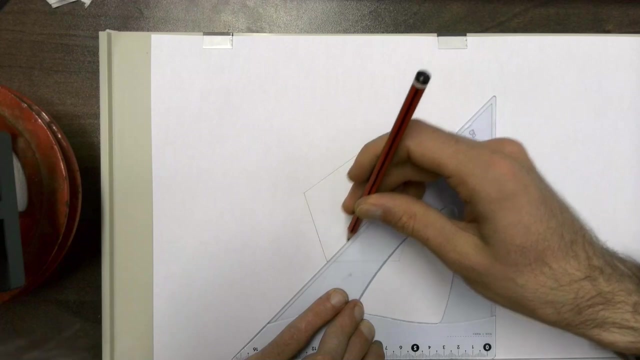 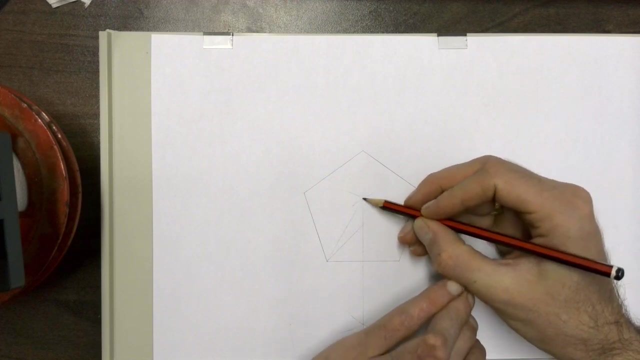 square, place it on the left base point of your pentagon and draw another arc. Take your construction line until it meets up with your bisecting line and then do the same thing with your 45 degree set square and then take the length of that line between. 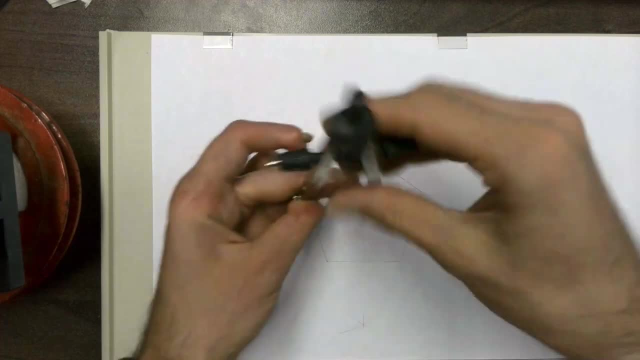 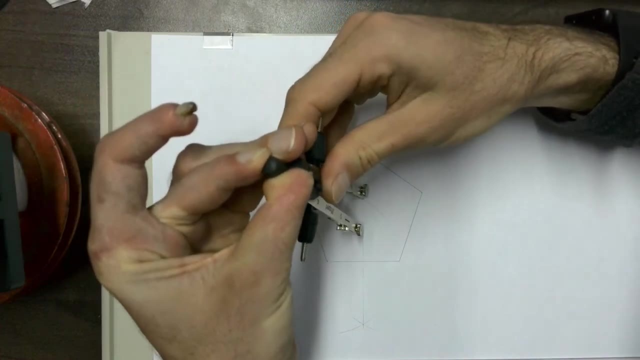 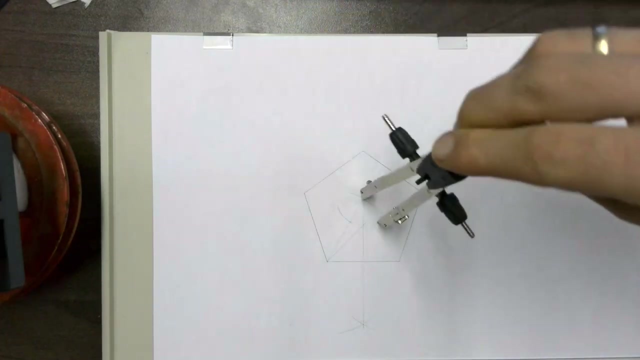 those two points and bisect it using the same method that we used to bisect the base: Placing our compass on that top point, Opening it up to the end of the line. draw an arc on the one side, arc on the other. 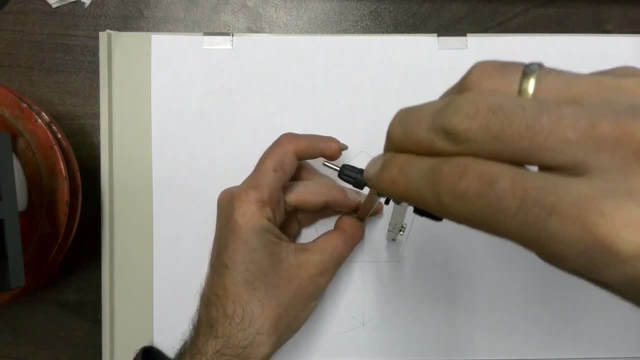 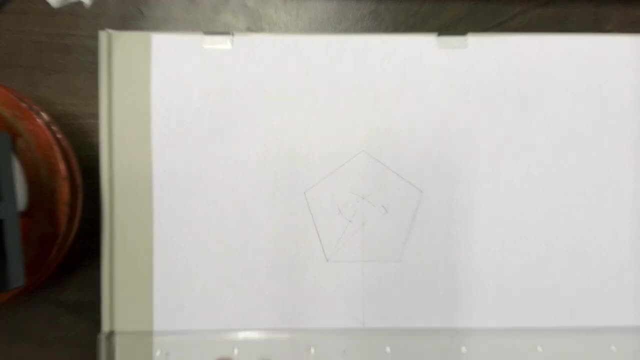 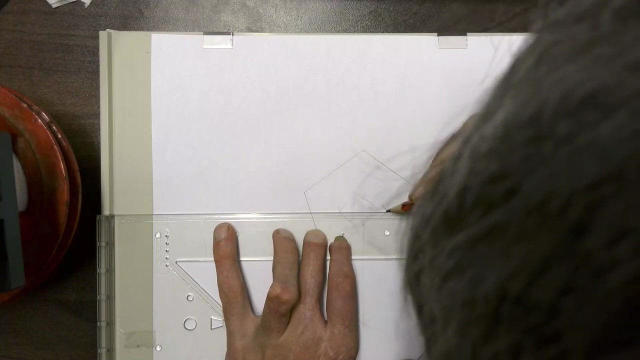 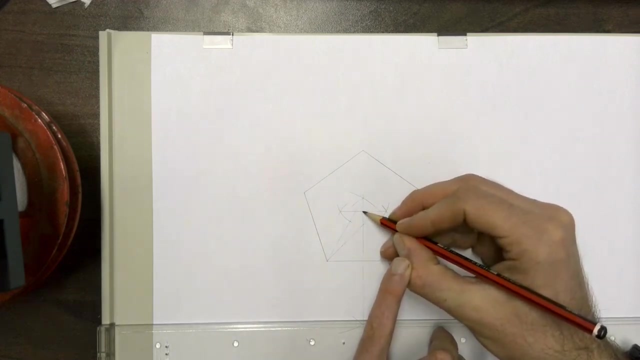 Flip the compass around, do the same thing on the other side- arc on the one side, arc on the other- and then go and join those two points where those arcs intersected, and then this point here would then be the center point of your pentagon. 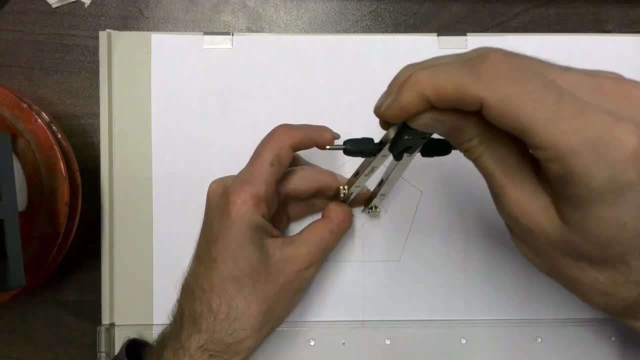 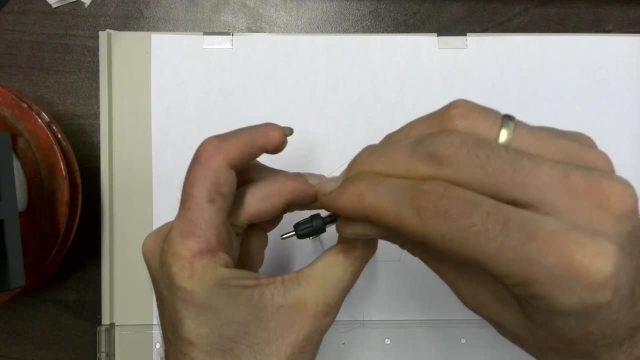 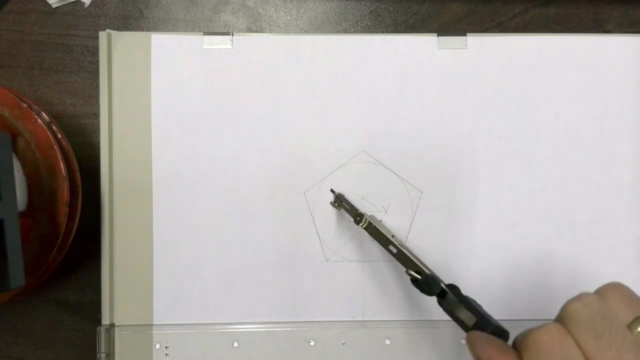 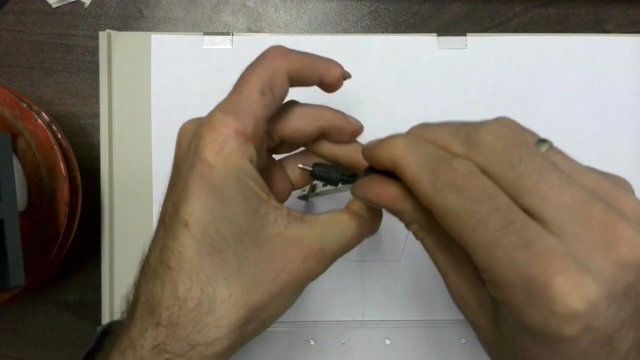 And if you take your compass, just check that, put your compass on that point. If you open it up to touch the one side of your pentagon, you should be able to draw an inscribed-circle which should perfectly touch each of the insides of each of the sides. and if you go right to Hiots, 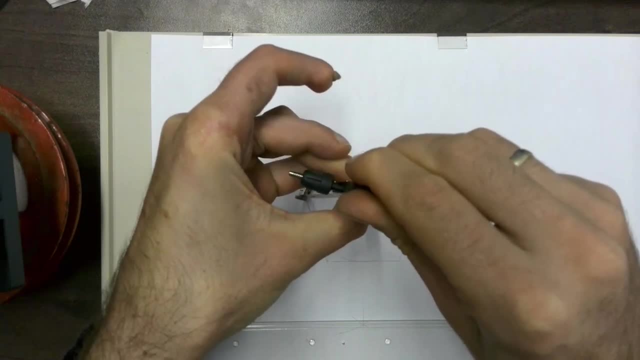 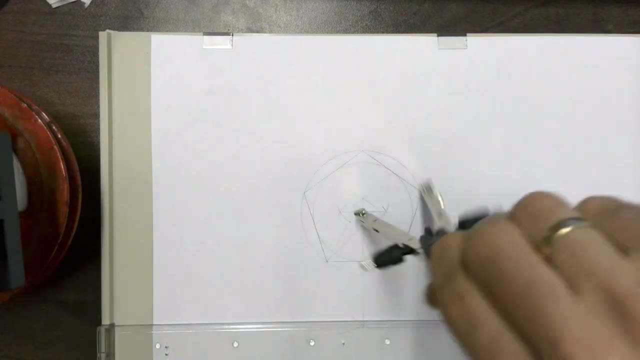 side to any of the corners, you should be able to draw another circumscribed circle which then should touch perfectly the outer corners of your pentagon.